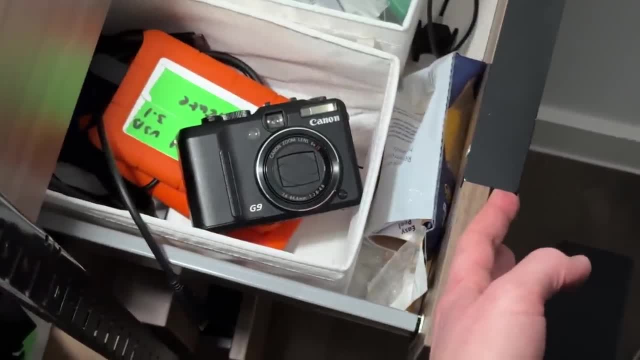 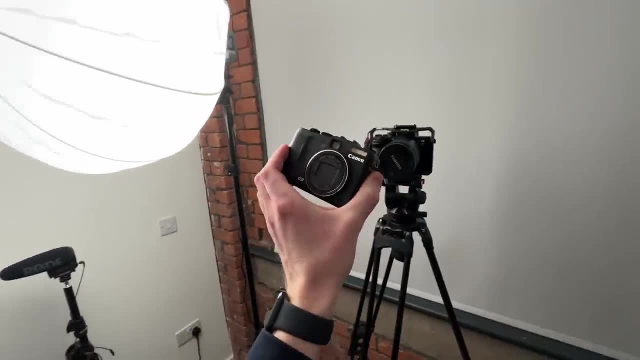 This camera actually belongs to my girlfriend's family, and only when we were visiting them did it get pulled out of the drawer. We both had a look at it, and then she ended up deciding to bring it home. Of course, I have then been stealing it to go out and shoot. 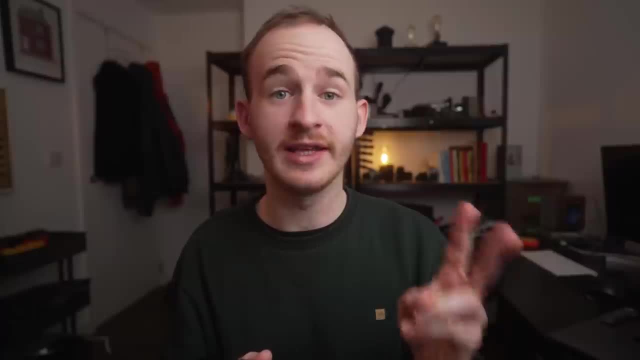 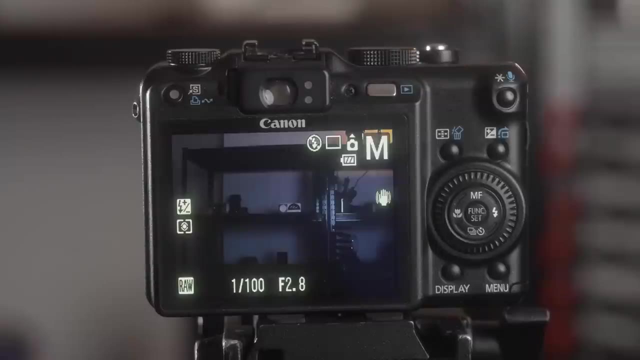 street photography with it. So in this video I'm going to do two very specific things. I'm going to give you my personal opinion on using this camera- the good parts about it, the obvious bad parts about it, I feel- And then also we're going to talk about the specs of this camera. 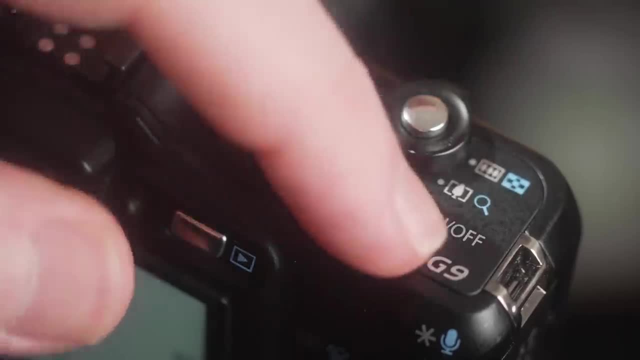 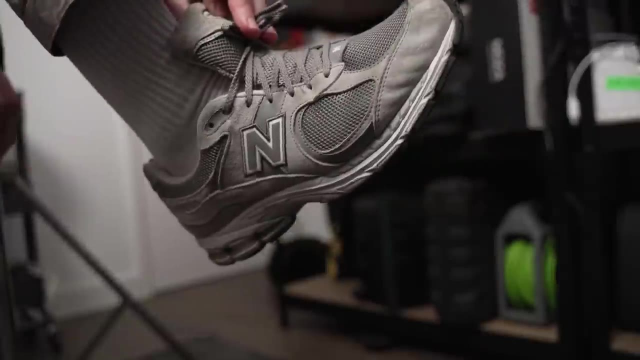 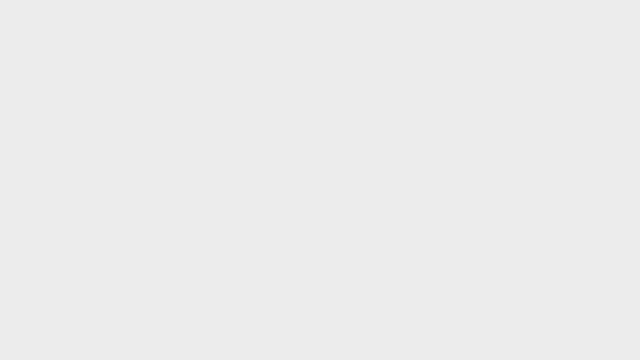 and why cameras of this age are probably worth investing in- if you find one in good condition- and just hold on to it for this kind of unique shooting experience. And of course, there's the added bonus to this camera being a certified dad magnet. All that aside, I'd like to talk about the 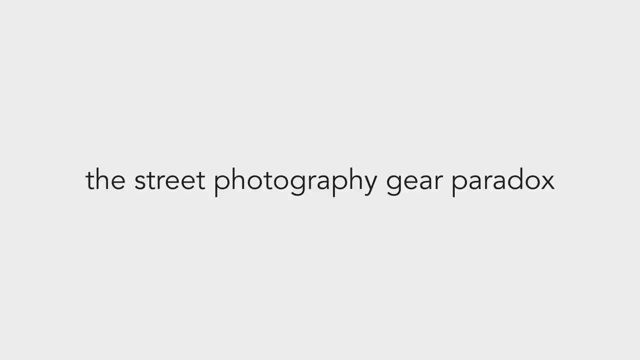 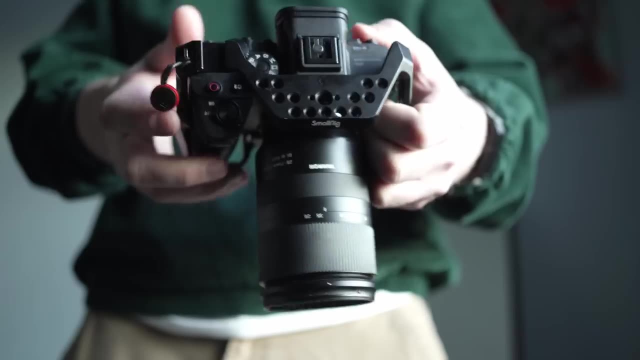 street photography gear paradox that I think we each find ourselves in. This is a journey that we each individually go on as photographers. as we explore street photography as a genre, We begin to acquire gear to, you know, do the job or to prevent errors mostly, And the little advantages. 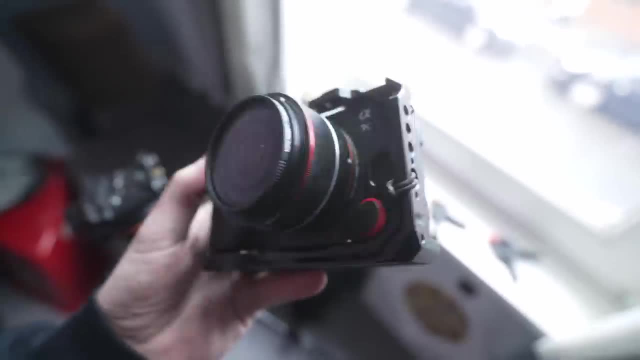 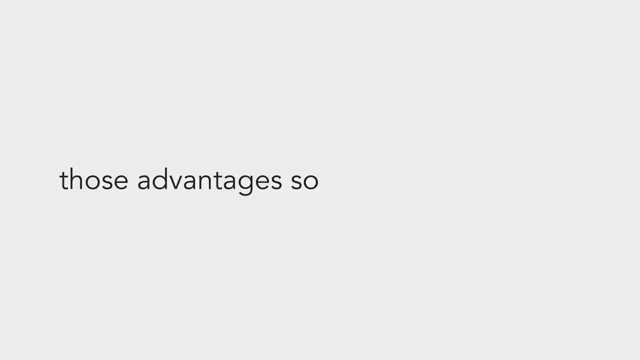 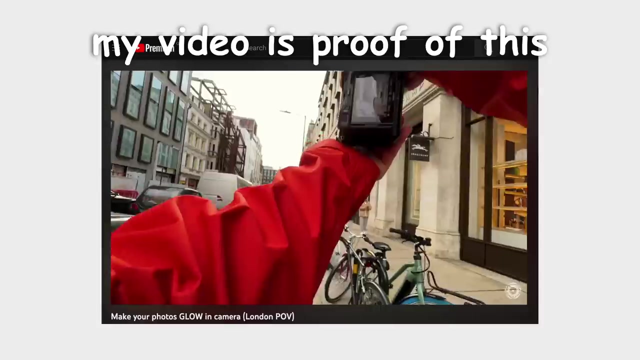 we get from, you know, better AF performance cameras, longer focal length lenses, constant f2.8 zoom lenses, etc. Those advantages soon turn into crutches, And then what was once the unlock inability that we get from a brand new mirrorless camera body and fancy new lenses soon become the 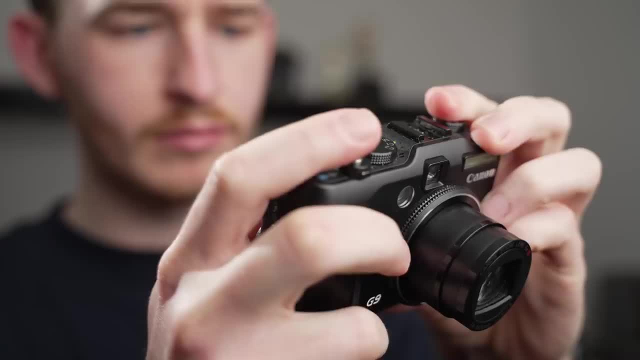 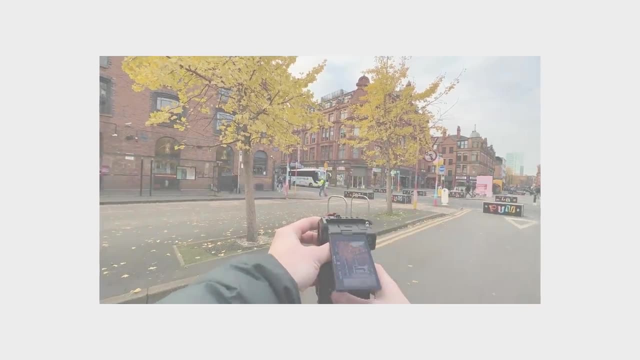 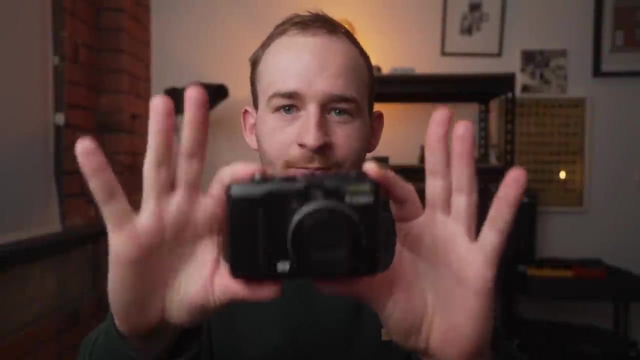 lazy option for practicing street photography And it removes a lot of the character, a lot of things that we're used to. Sometimes that lack of risk actually makes taking photos unexciting, And that leads me back to this little doodah that came out when I was 11 years old And there is so 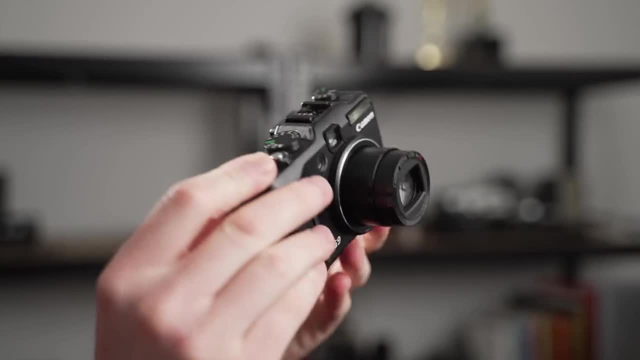 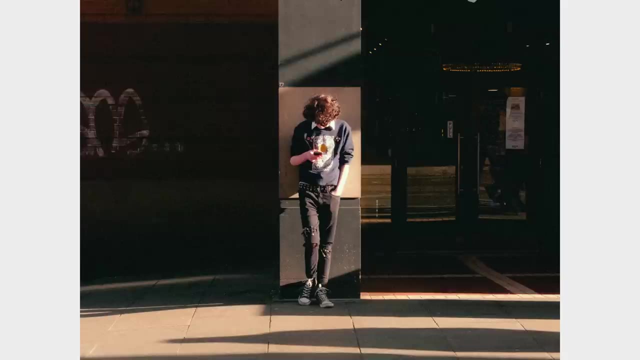 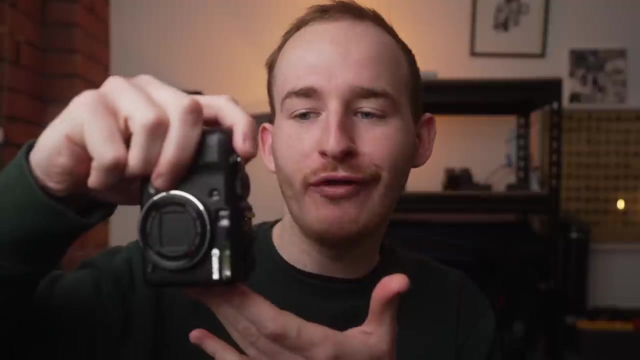 much wrong with this camera that makes it so much fun to actually use when shooting street. And there's so much about this camera that just takes away any of the shallow depth of field decision. You know it takes away any of that. Oh, what setting should I use on my camera to get the right photo? 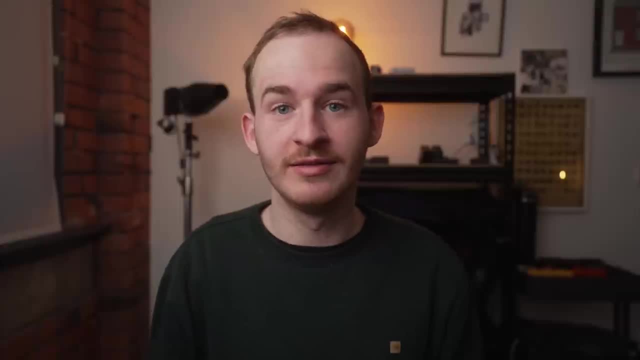 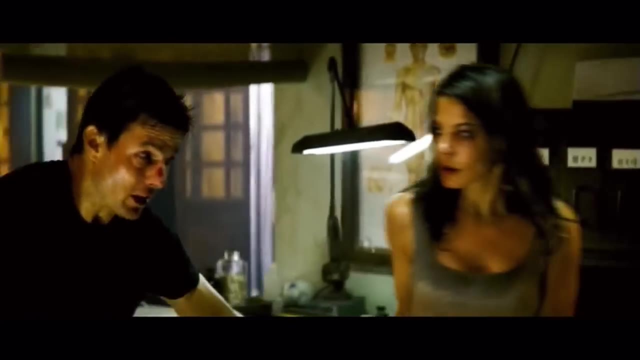 There isn't that. You just just point and shoot, mate. Point shoot, point shoot, Like Tom Cruise in Mission Impossible 3.. Point shoot, Point shoot. Very simple, Point shoot For a compact camera from 2007,. 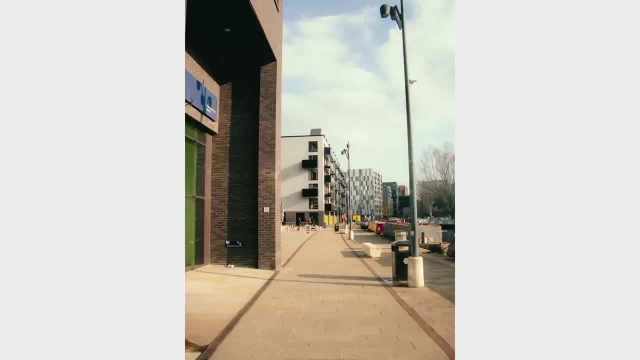 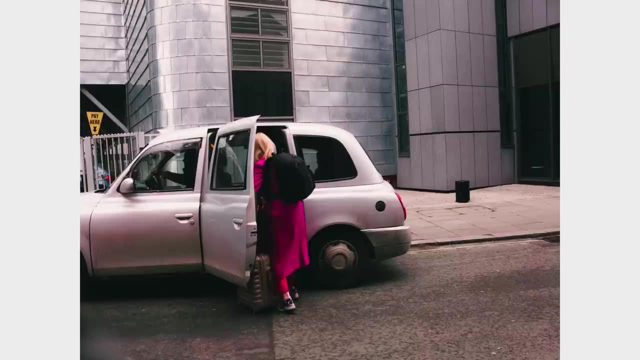 this PowerShot G9 provides really nice high quality raw images of 12 megapixel resolution And it shares a common trait with a lot of cameras from like the mid 2000s of having a CCD sensor rather than, more commonly today, a CMOS sensor. 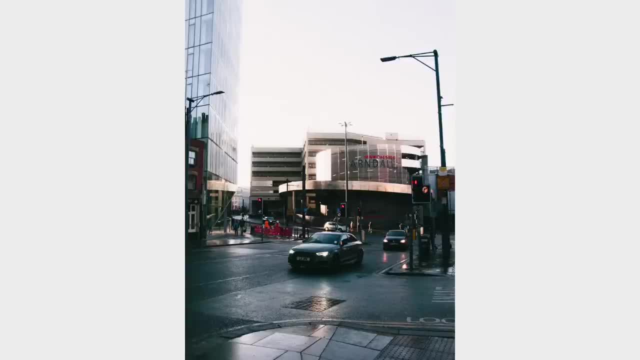 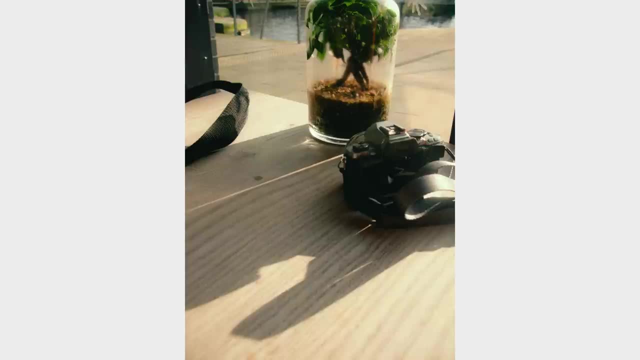 Although these images come from a smaller sensor, the combination of the CCD technology with the built in lens and then also the pixel density on a sensor like this actually provide us with really pleasing soft images At a glance. looking at the raw images, they are very flexible and of high 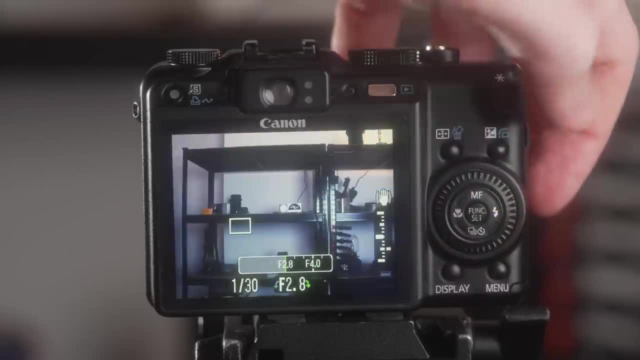 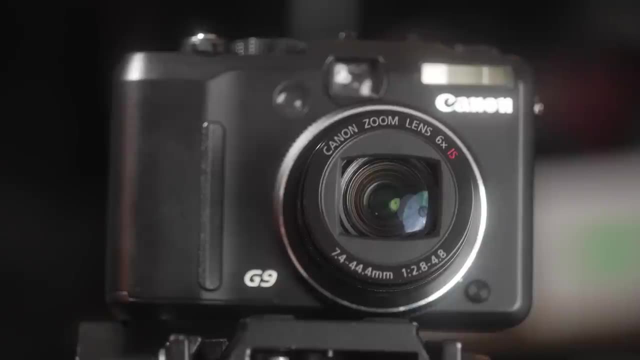 quality as long as you get your metering right in camera. The lens provided actually gives an optical zoom of 35 millimeters up to 210 millimeters, And while I'm rarely zooming in that much on this camera, I have taken the 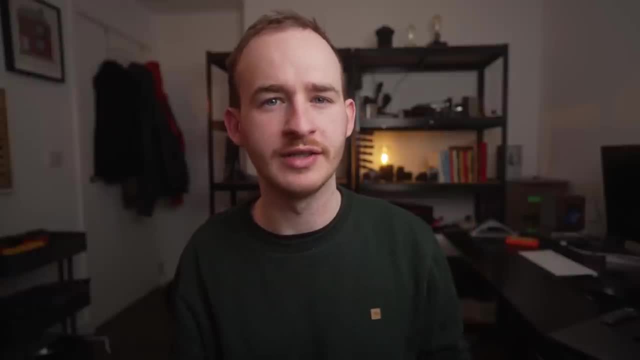 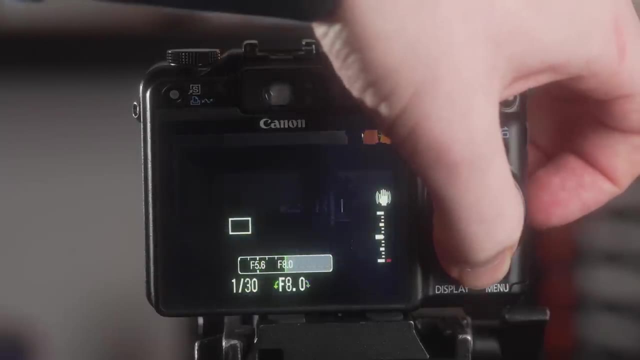 large one at about 50 millimeters and sometimes around 100.. But for the most part I'm powering it on and shooting at the 35 millimeter The widest aperture is actually an f 2.8 and the smallest aperture is actually an f 8.. But to compensate for this they have also 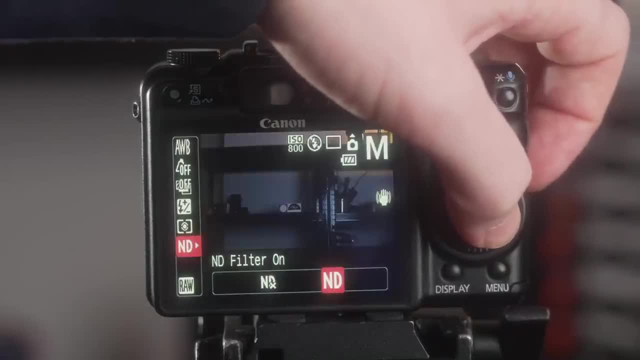 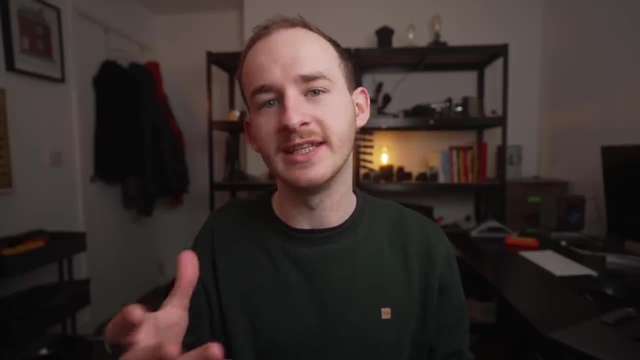 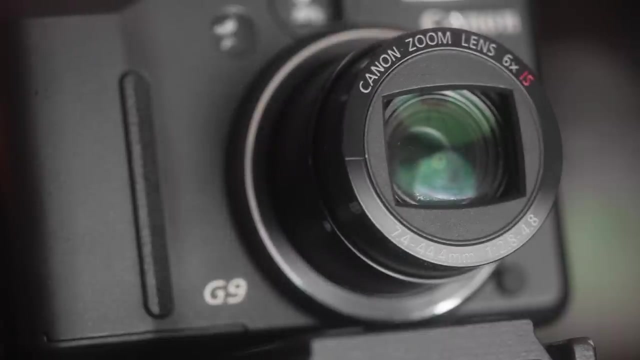 included an ND filter within the camera to help balance on those brighter daylight days. The lens itself is actually the place that I was surprised by the quality the most. I have mixed feelings about what it can do. It is an optical zoom up to 210.. So it means that you have higher quality. you're not sacrificing anything with digital zoom- sort of to be expected from the. 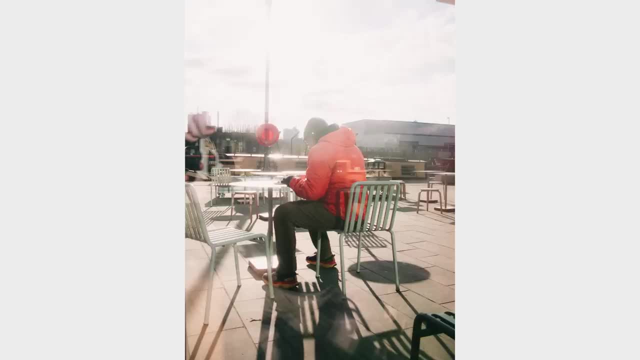 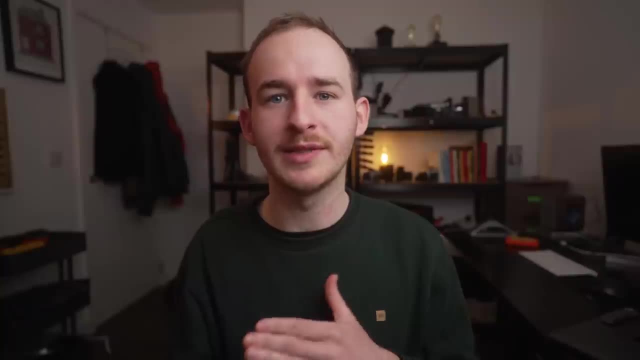 PowerShot, more pro compact cameras. But this problem with the lens can actually lead to quite a nice feature, and that is seeing some highlight bloom in certain areas, And when I've been shooting with this camera sort of at the same time as my Minolta, I then look at images. 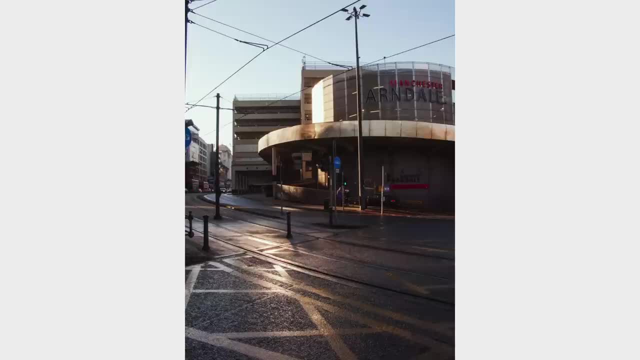 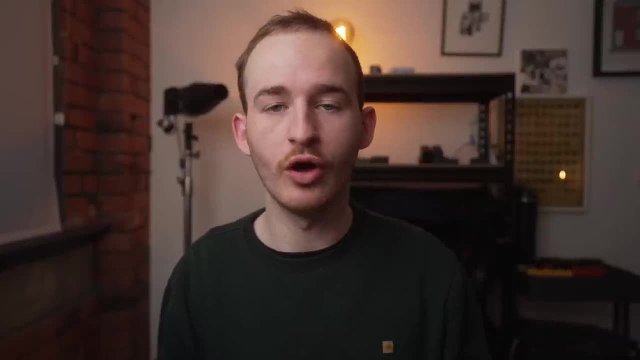 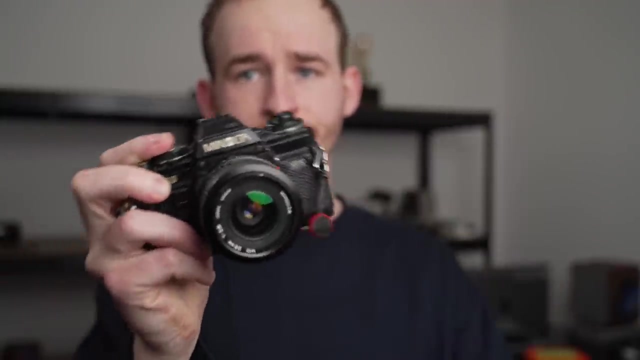 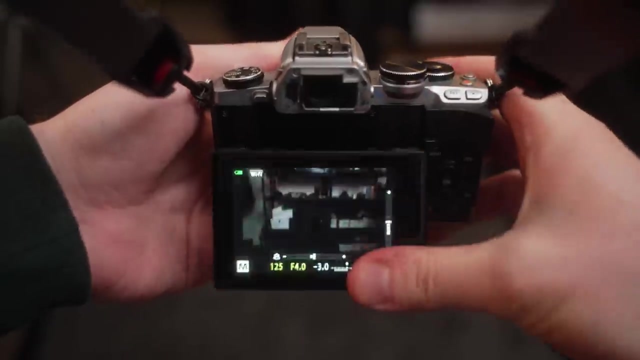 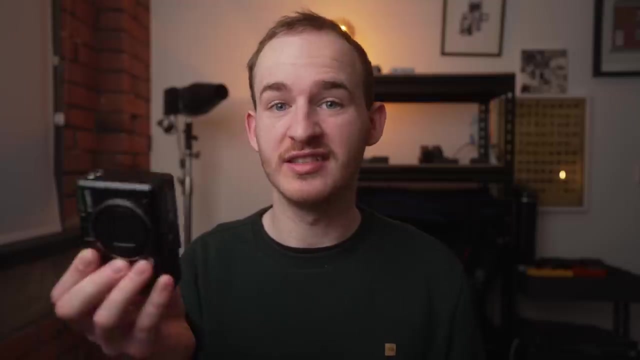 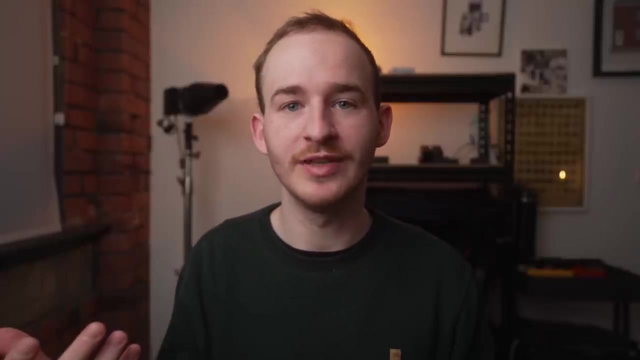 afterwards. I think, hang on, I'm getting kind of a similar play with highlights here, without having to use something like a diffusion filter. I have been primarily using this camera during the day on photography walks, when I've been using either my 35mm, Minolta X700, and I'm either trying to save shots on a roll of film or I finished a roll of film. this has been in my pocket ready to go, but I've also been carrying it with me when shooting with, say, my Olympus E-M10 or my A7C, just as an extra little break if I feel like I'm kind of doing the same thing with my interchangeable lens camera that has more flexible features and better up to speed. 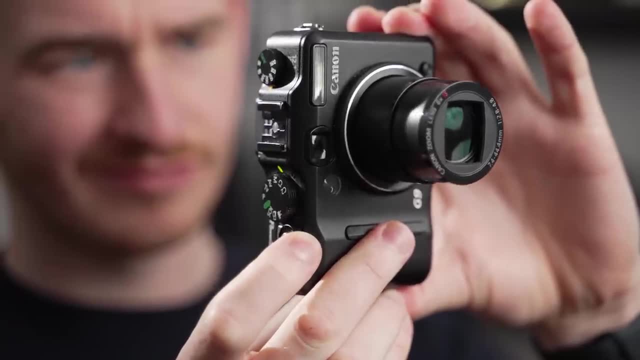 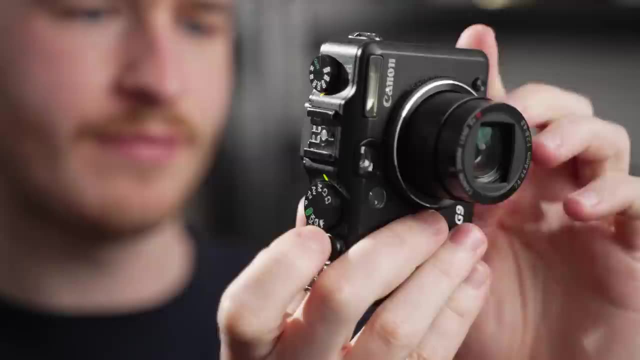 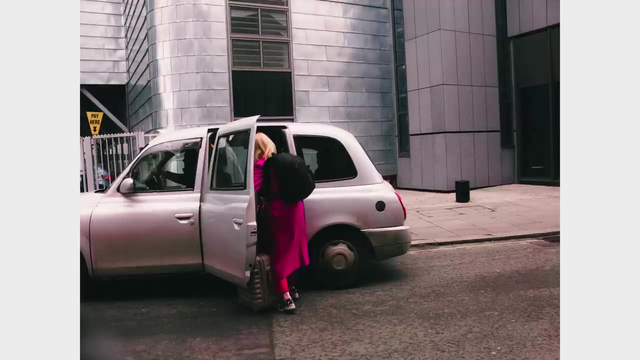 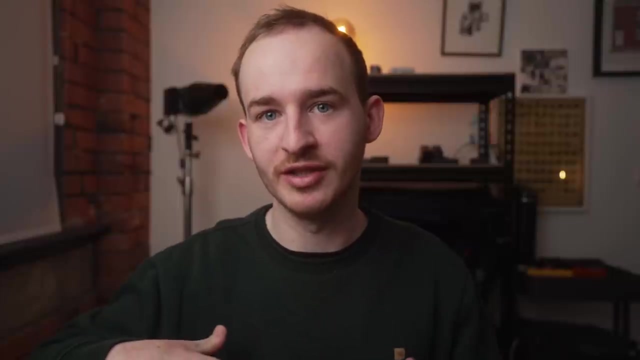 Optics, I feel like I'm getting the same results. I'll pull this out for 10 minutes and it kind of cleanses the palette in terms of what you're looking for with your perspective. A lot of the shots I've been taking on this camera have been more like locked off scene shots- odd candid shots- but really what I've been seeing at the end of the day is it makes me think about my position, like my physical position in relation to the subject and the scene as a whole, a lot more than shooting a lot of shots. 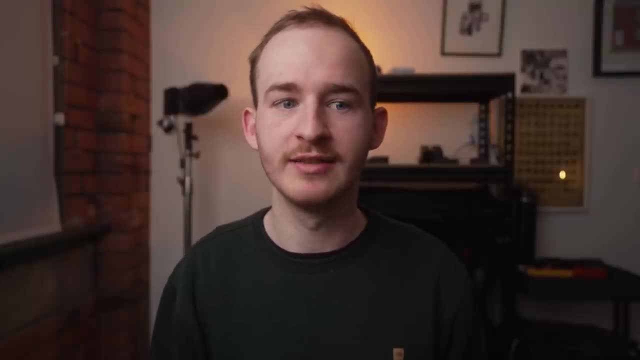 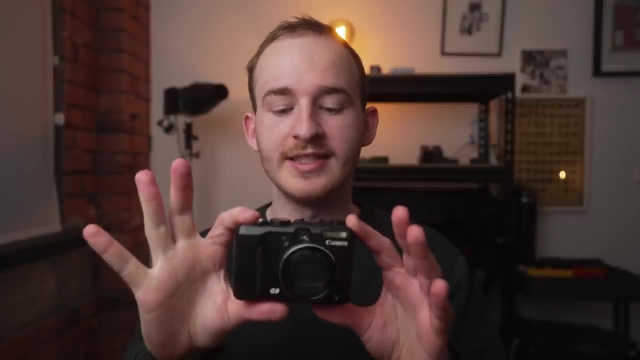 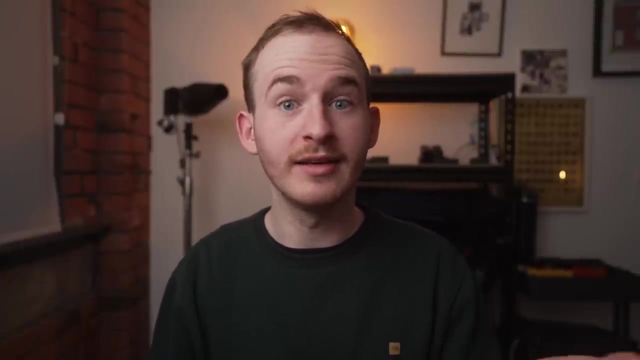 If I'm shooting on something with a longer focal length or more flexible optics or something where I'm kind of a bit more worried about being seen taking a photo with a larger lens, for example, this definitely removes a lot of that and allows you just to focus on making a photo that you like. 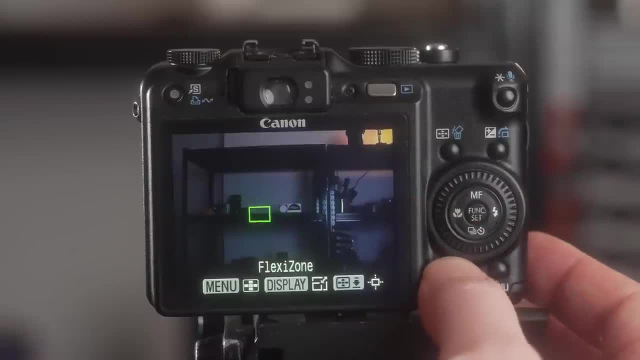 The autofocus system on this camera is really nothing to write home about. So we have face detect autofocus. I haven't used because I've been doing street. We've got AI area autofocus, which is pretty good. It's pretty much just the center of the screen anyway. then you've got this flexi zone and I've been mainly using the flexi zone, but I just push around a little bit. 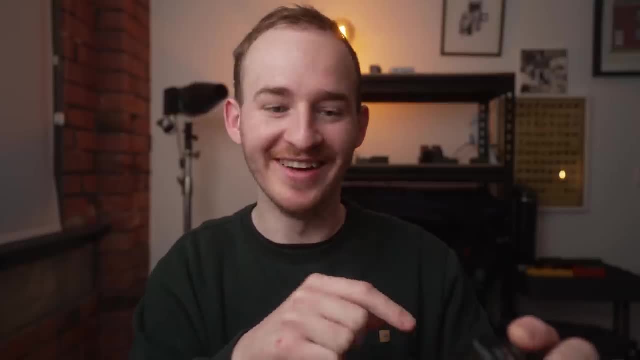 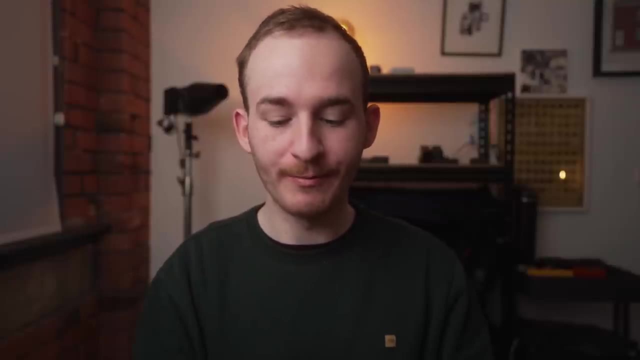 Like if I see something happening, I'll move it to that part of the monitor then get that in the frame. but it's really, really rudimentary and there's something about that that just removes any of that thought process. Like you know, I hadn't even really looked at that and I've been using this for about a month and I've been really happy with a lot of the images I've been taking. 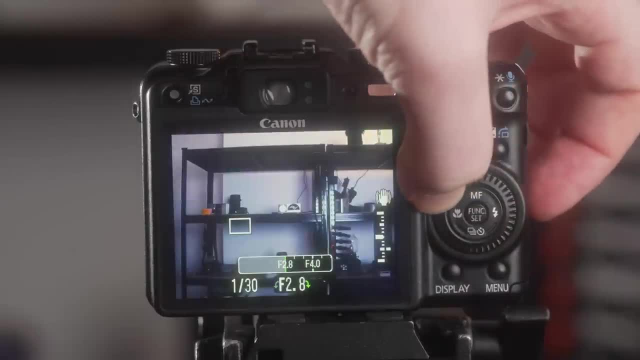 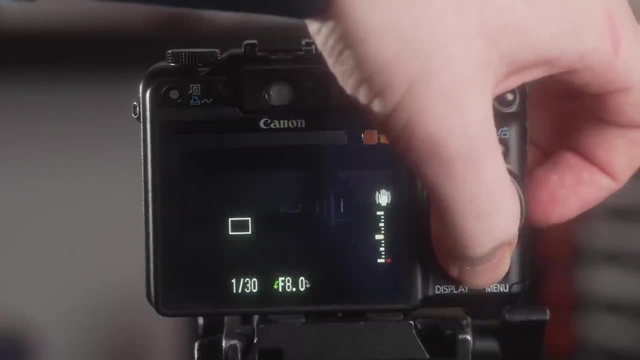 One of the biggest problems with this- that I definitely this is actually a very serious problem- is the screen brightness and the actual dynamic range of the display is really not to be trusted if you're using it to sort of exposing your images. So it's really important that you actually pay attention to the meter. 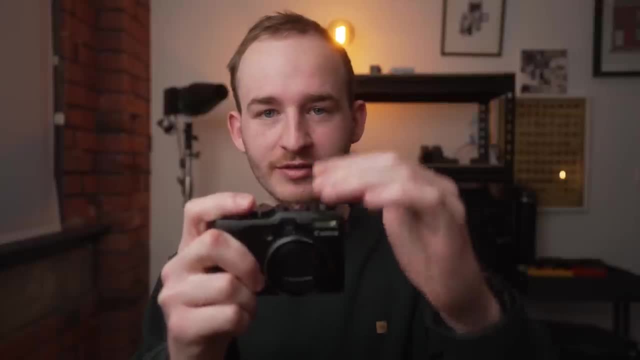 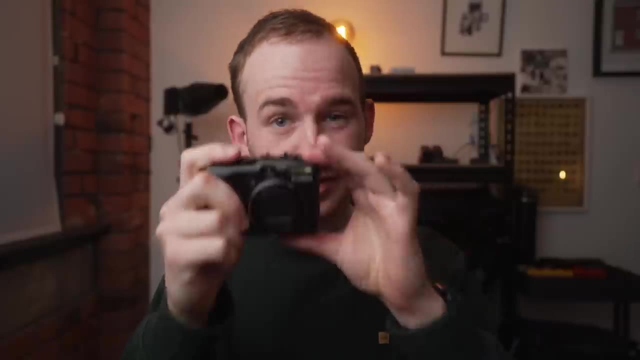 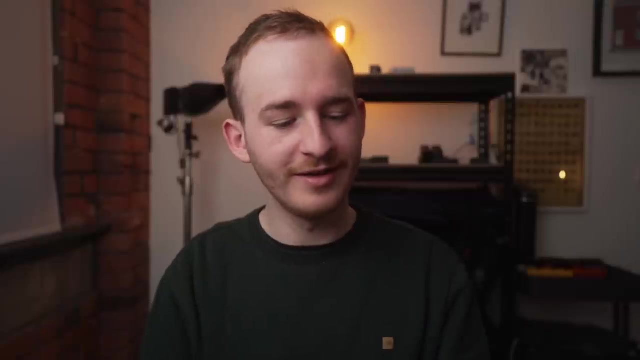 We do also have a little OVF, like you know, a little kind of like not rangefinder, but you know the old disposable camera style OVF and it's tiny when you look down, So you can use that on like a bright day just for framing something, but it feels a little bit silly. 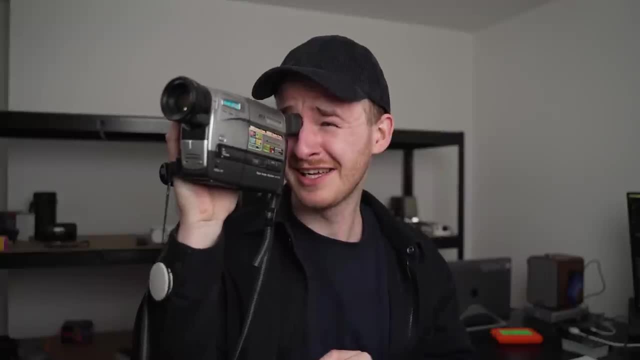 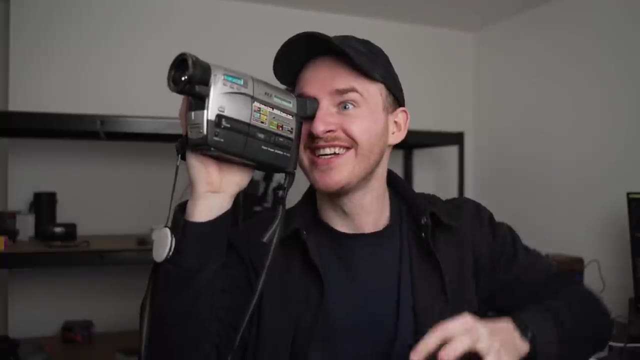 I can't say I've been using that very much. Get your VHS camcorder in one hand, your PowerShot in the other hand, and now you've got everything you need to either make an indie film project at university or document it out of your kid's school play. 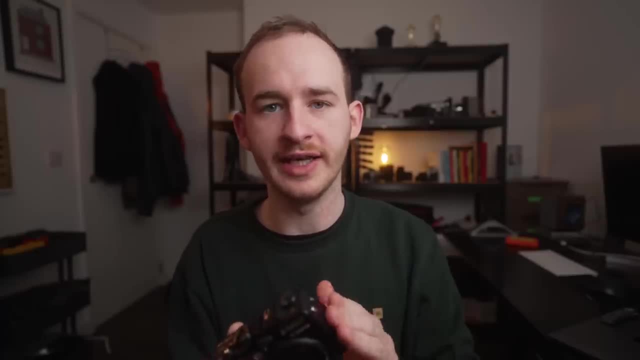 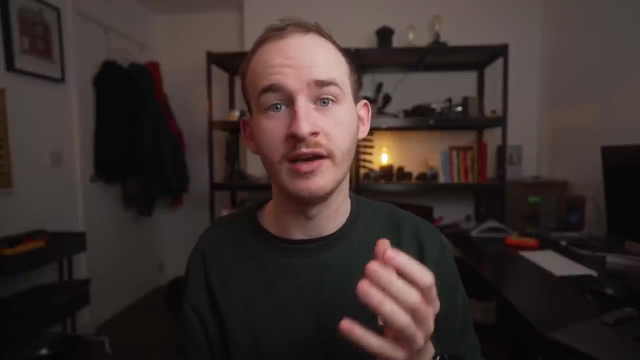 As I have briefly touched on already, the heart of this camera is a CCD sensor which, if you don't know, is a charged couple device Versus what we get today in most cameras, Which are variations of a CMOS sensor, which is a composite metal oxide semiconductor. without getting into the nitty-gritty of what differentiates a CCD sensor from a CMOS sensor and also why we don't really see any new CCD sensors today, 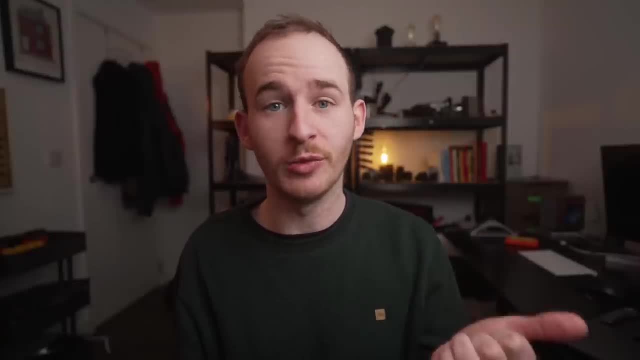 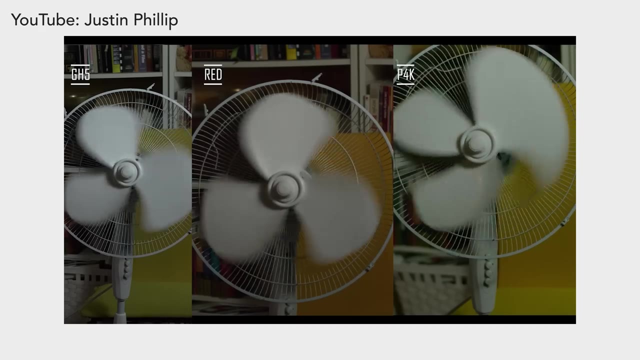 One of the main things you need to know is that CCD sensors use a lot more power inside the cameras to record photos and they are also more expensive to produce. One of the main advantages of CCD sensors that you will have seen in camcorders of the past is the fact that they're not as expensive as they used to be. 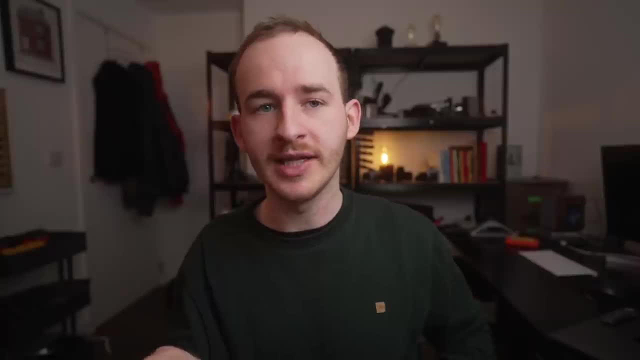 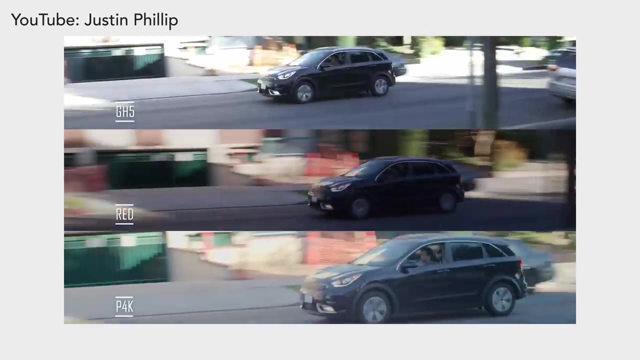 They actually operate what is essentially a global shutter, meaning that every single pixel on the sensor records at the same time, meaning you don't get that kind of jello effect rolling shutter when you film using a digital camera that you might see on, like Sony mirrorless cameras, for example. 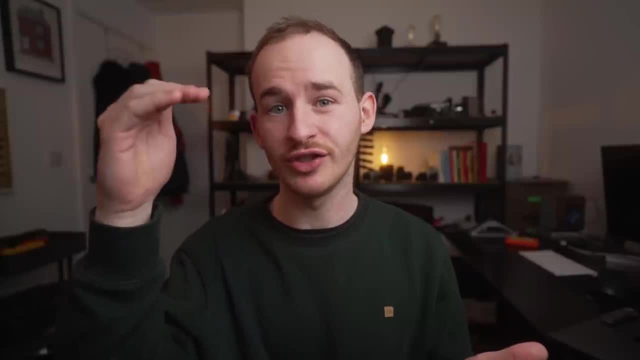 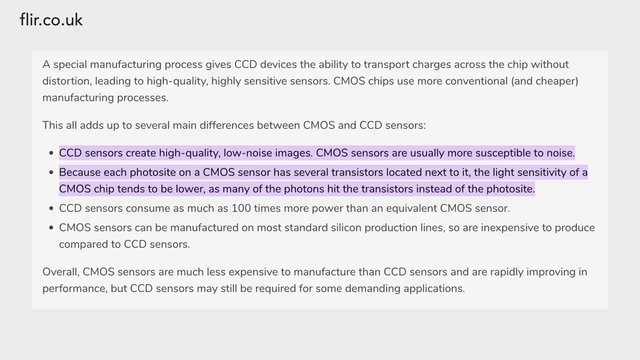 This is in contrast to this CMOS sensor, which is actually a rolling shutter which records row by row, preferably as fast as possible. The main reason why CMOS sensors were chosen over CCD Because they were cheaper to develop. so we've been able to advance the technology with cheaper development upfront, versus manufacturing expensive sensors that were kind of already good. 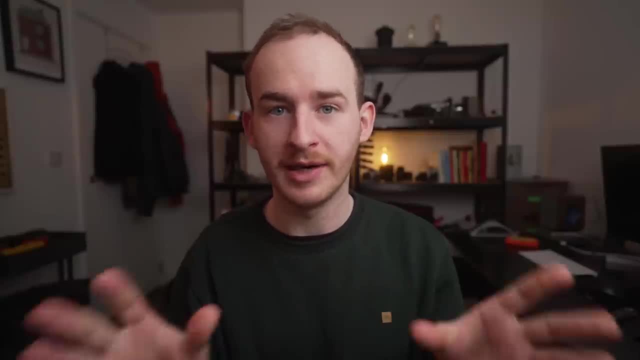 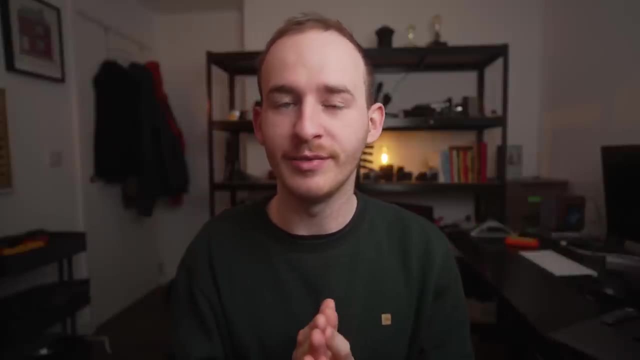 I understand people who may know more than me on this matter might have other opinions or other facts that I've missed out or got wrong. I'm going to drop some sources in the description below. This is to the best of my knowledge, but please do your own research if you want to be able to impress your friends at the pub. 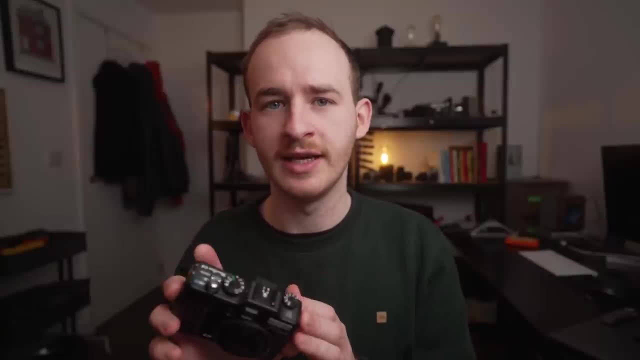 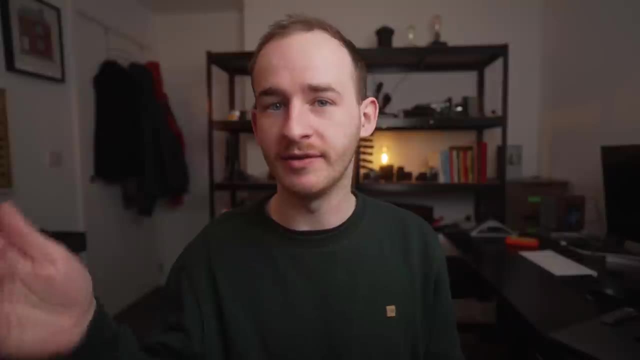 I also mentioned previously that this is a 12 megapixel sensor And while that might seem like a lot of money, it's not. And while that might seem like a lot for a compact camera, which it kind of is, compact cameras today are getting to 20 and above in megapixels. 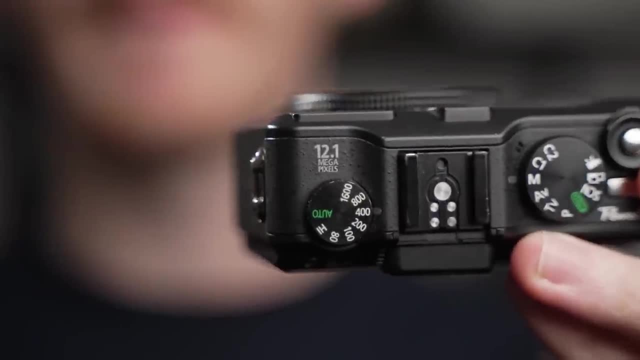 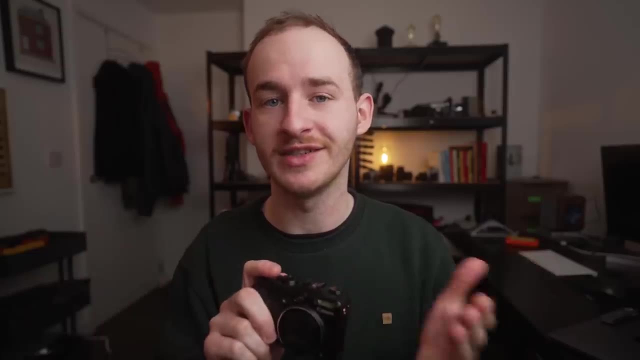 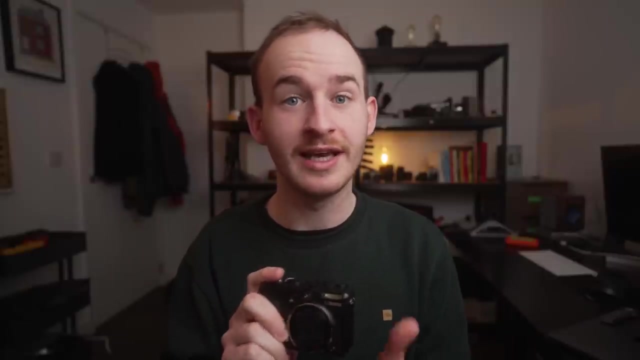 But there's also compact cameras from about two years before this that have got one quarter of this megapixel count. There is a trade-off when it comes to how many megapixels you pack onto a sensor of a certain size, And 12 megapixels on this size with this technology of CCD versus CMOS is definitely a sweet spot.